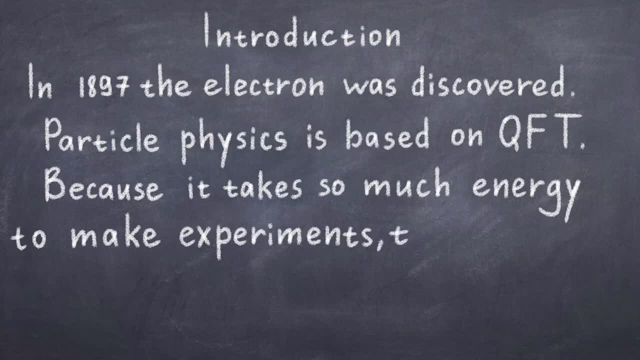 Today, physicists all over the world study this field, at least theoretically. Because particle physics takes place at scales below a nanometer and experiments require a lot of energy, it is only possible to make experiments at a few special places around the world. One of the most famous places for particle physics is at the Large Hadron Collider at 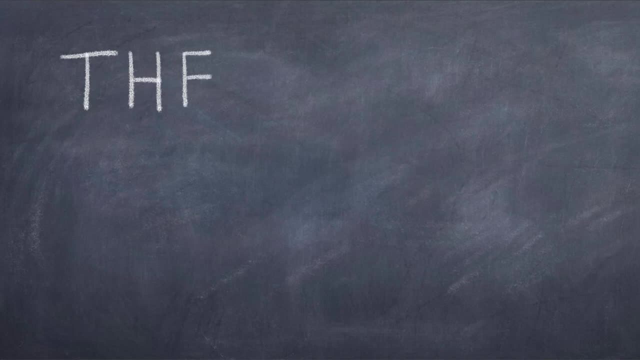 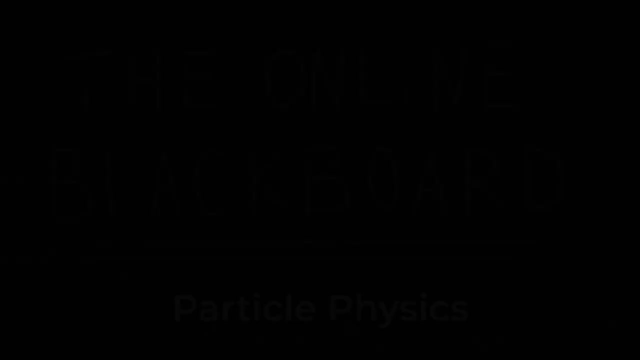 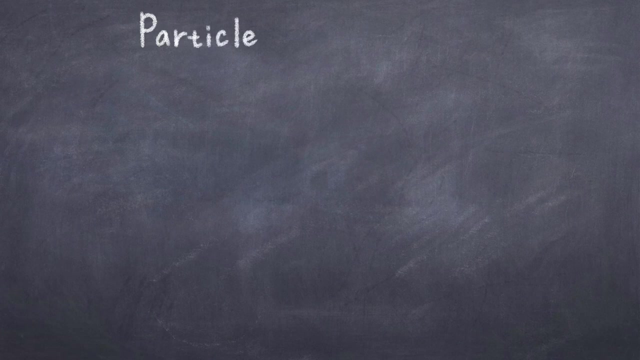 CERN in Geneva, Switzerland, The field of particle physics quickly began to take shape in the 1930s from the ruins of the classical world. After the formulation of quantum mechanics around 1923 to 1926, the interest in quantum physics increased. 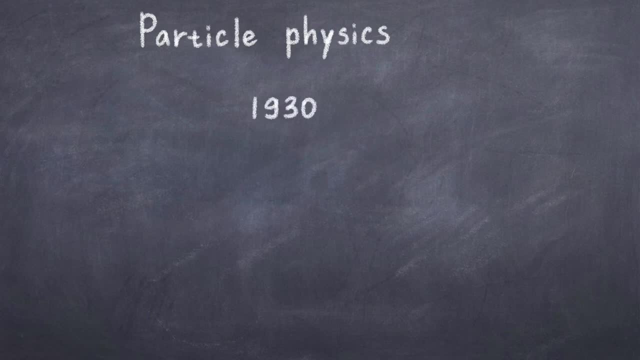 The next step was to formulate relativistic quantum theory, which we now know as quantum field theory. In 1927, Paul Dirac came up with the first relativistic quantum equation, called the Dirac equation. It turned out that this equation predicted antiparticles. 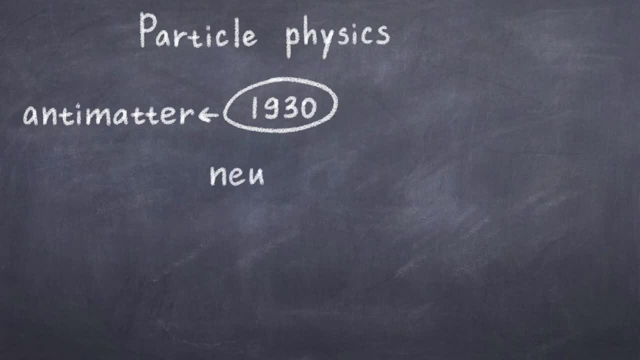 This led many to believe that the equation was false, as such particles were not known to exist at that time. This, however, changed in 1931, when the positron, or antiparticle, was discovered. The positron was the first quantum equation to be discovered in the world. 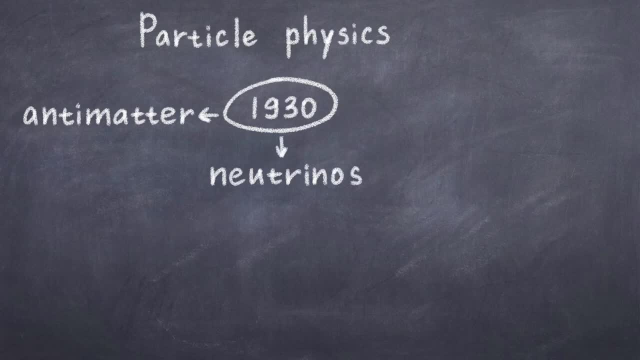 It was the first quantum equation to be discovered in the world. The second quantum equation was the first quantum equation to be discovered in the world. The third one, called the antielectron, was discovered. The issue of how the nucleus could be stable with a positively charged proton was resolved. 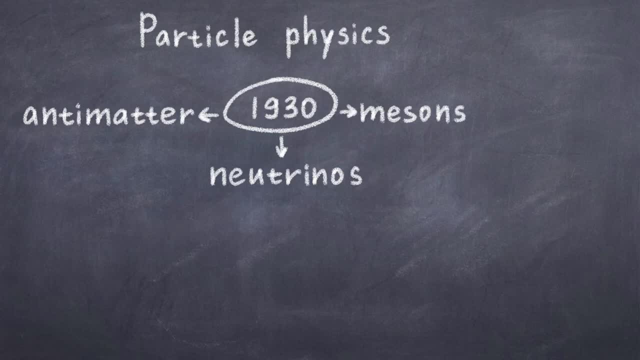 with the prediction of a new particle. This new particle, later named the pi-Mason, was the first of a new class of particles called Masons. In the meantime, in the 1930s, people were puzzled about what actually was going on in. 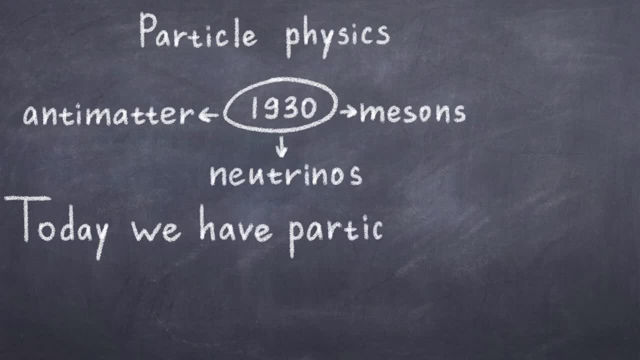 beda decays, and this eventually led to the introduction and discovery of neutrinos. After the discovery of the pie mason, it was thought that particle physics was more or less well understood, And now we know that they were only getting started on particle physics. 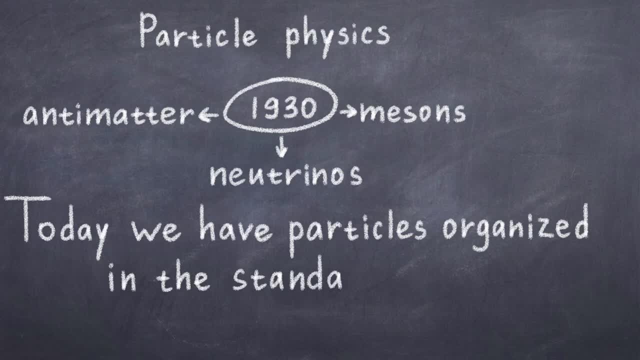 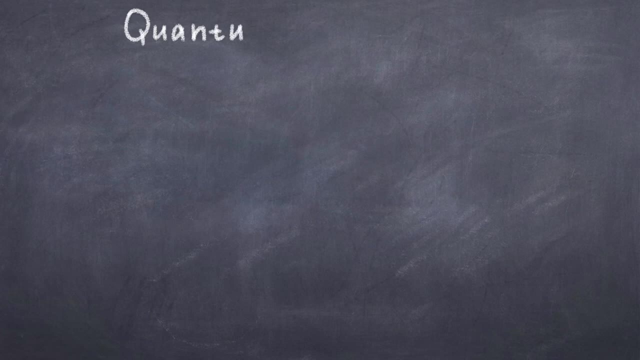 In the following years, many new particles were discovered, and the relationship between the particles was only understood much later with the invention of quarks and the standard model, and eventually we got to where we are today. In particle physics we use Feynman diagrams to describe different processes. 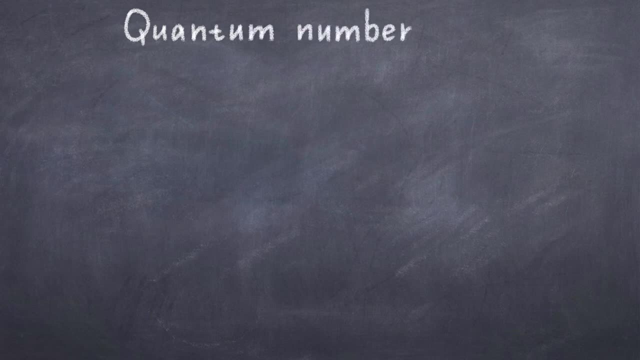 However, things are a bit more complicated in real life than in the toy model which we considered in the video about Feynman diagrams. First of all, in the real world we have a lot of particles to work with and we can't just put any particles together. 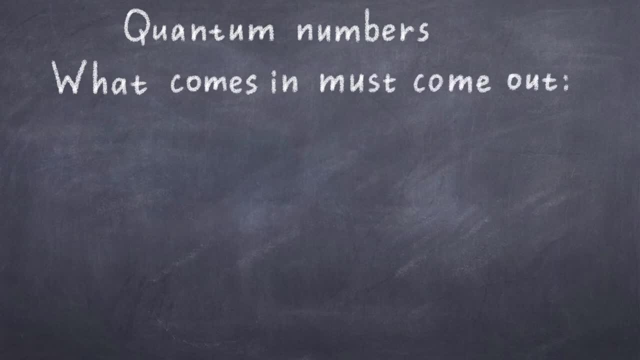 The key to figuring out what is allowed is conservation of quantum numbers. What comes in must come out. As discussed in the video about the standard model, we have three fundamental forces to work with. in particle physics We have the electromagnetism, The magnetic force. 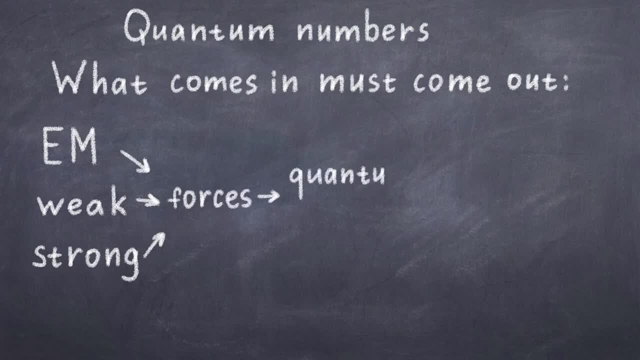 The weak force And the strong force. We will see that the weak force is a bit special. In order for us to make a valid Feynman diagram, we must conserve the following quantum numbers – charge, color, barrier number, lepton number and flavor. 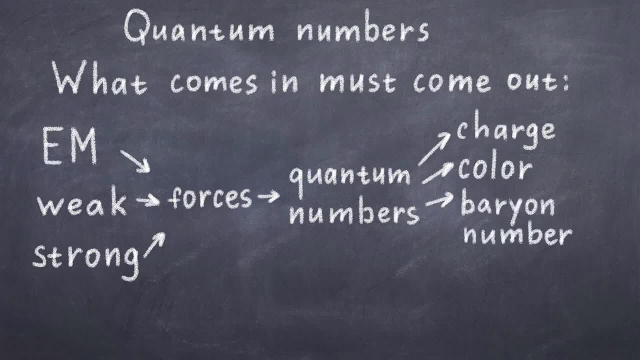 The latter two, however, comes with an asterisk. Lepton numbers may be a mix between generations. in some special neutrino oscillation cases, The flavor quantum number is not conserved by the weak force, As it generally changes flavor. This means that the identity of particles can be changed like an up quark changing. 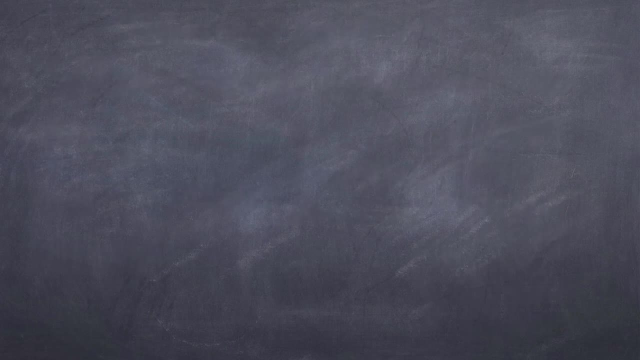 into a down quark. Let us consider in more detail what it means to conserve charge and color. In Feynman diagrams of real particle physics we denote fermions or matter with a solid line with an arrow. The arrow is to show the fermion current. 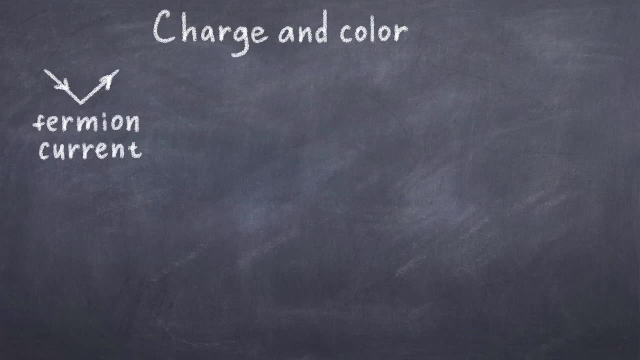 If it goes forwards in time it represents usual matter, But if it goes back in time It represents antimatter. This flow must go one way And this actually also conserves the fermion number of any process where antimatter has minus one and matter has plus one fermion number. 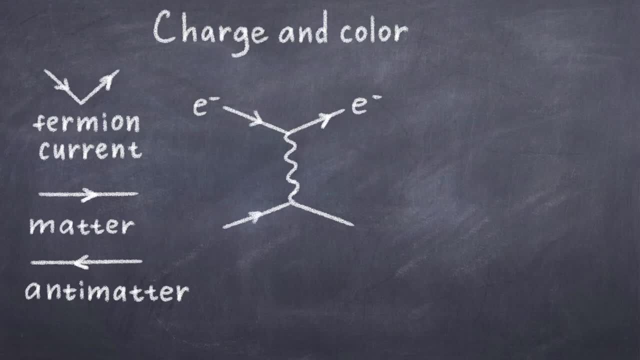 Now let us go back to charge conservation. A simple process to consider would be the repulsion between two electrons. We have two charged electrons coming in and then they interact via a photon and then go out. We thus end up with two electrons interspersed. 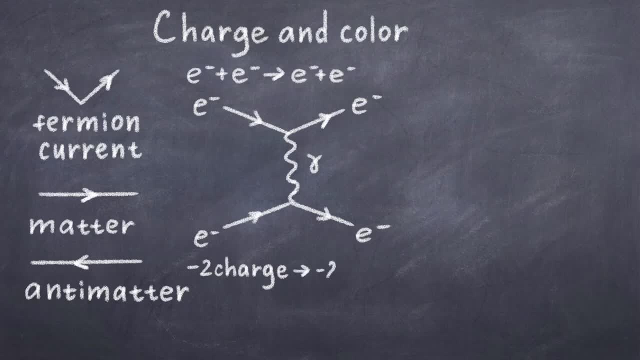 We have two charged electrons coming in, and then they interact via a photon and then go out. We therefore have a charge of minus two before and after. Now let us consider the conservation of color. This is sort of a charge associated with a strong force. thus it is only relevant for 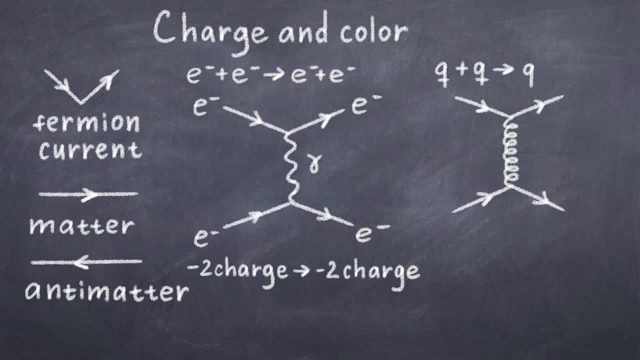 this force. We have three colors: red, blue and green- and the anti-colors of that. Only quarks have color. So we can consider the case with two incoming quarks which interact via a gluon. Let's say one quark has a blue color and the other has a red color. 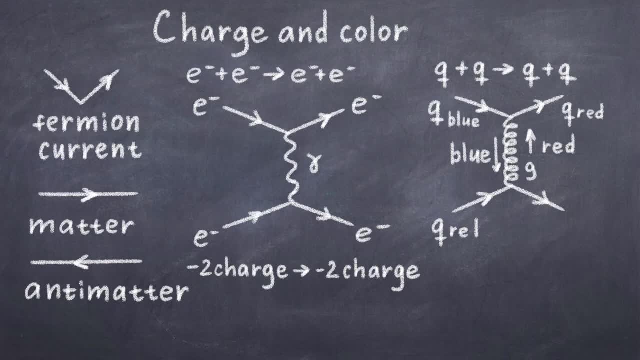 The gluon can contain two colors, so the gluon will be blue and red. When the particles interact, the gluon will thus carry the red color to the blue particle and the blue particle gives its blue color to the red particle. We thus have that the particles swap color. 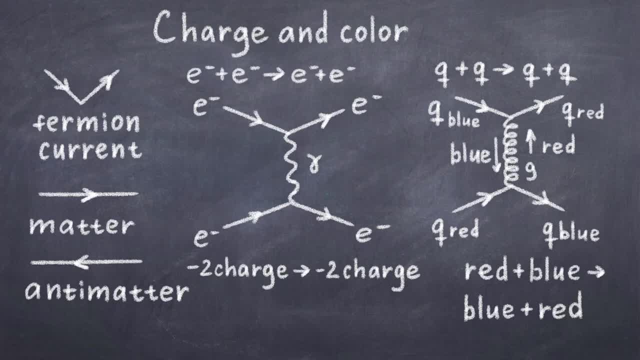 But color is conserved, as we still have blue and red color before and after. Next let us consider baryon and lepton number conservation. The baryon number of a baryon is the number of electrons. The number of electrons is the number of electrons. 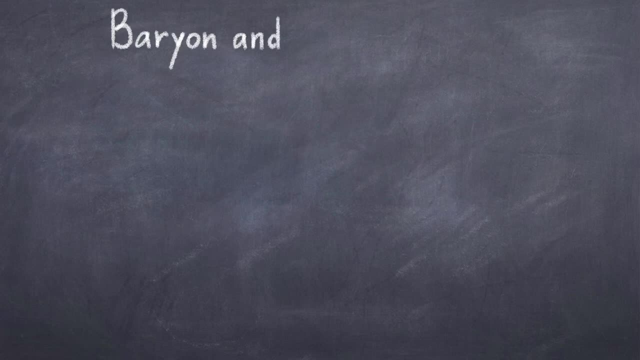 The number of electrons is. the number of electrons like a proton is 3, as it contains 3 quarks. Likewise, antiprotons have a barrier number of minus 3 as they contain 3 antiparticles. Mesons which are made from quark-antiquark pairs therefore have a barrier number of 0. 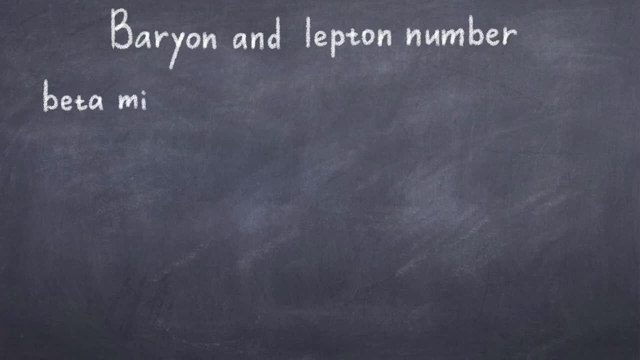 which means you can make a lot of them in a reaction, as they don't affect the barrier number conservation. An example of barrier number conservation is the beta-minus decay. In this case you start with a neutron which is made from two down and one up, quark, and therefore you have a barrier number or three, One of the down quarks turned into an up quark, turning the neutron into a proton. This is a flavor change caused by the weak force, and we also end up with an electron and an electron antineutrino. From the point of view of barrier number conservation, everything is great. We start with a. 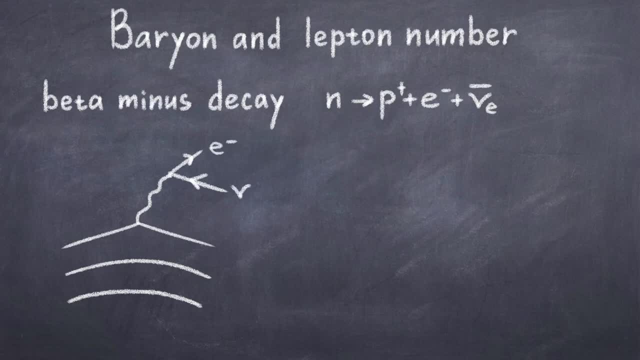 neutron and end up with a neutron with a proton, and both has baron number 3, so things are good. Now the situation with lepton number conservation is more interesting. This decay was exactly what led to the prediction of a neutrino. 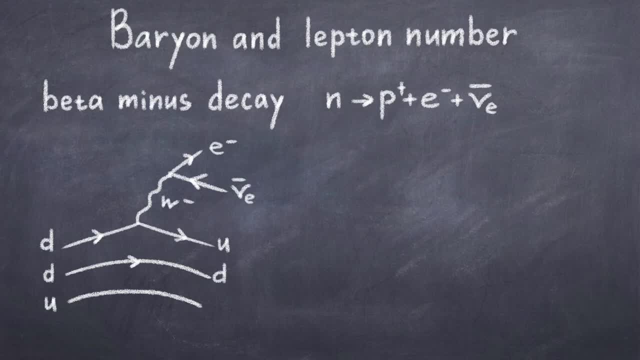 First of all, this process only matches experimental data if there is a neutrino to give us the correct kinematics. But we can actually see that the lepton number conservation also demands that the neutrino must be there In the beginning of the process. we only have a neutron. thus we have lepton number 0. 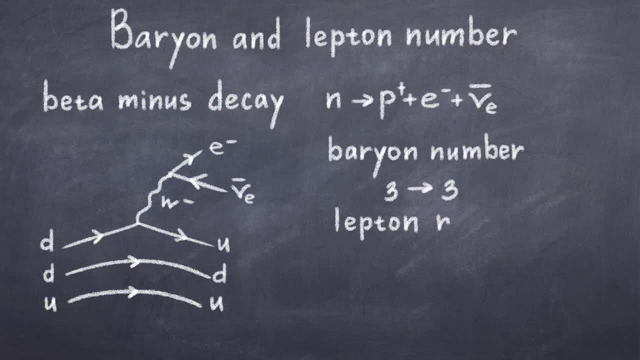 But if we only had the electron afterwards, we would have a plus 1 lepton number. Therefore we must have an antineutrino to cancel this out. So with the antineutrino we get: 1 minus 1 is equal to 0, and lepton number is conserved. 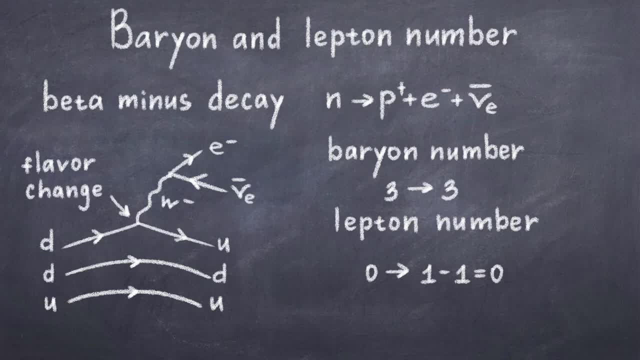 This process is also an example of how flavor is broken by the weak force. The W minus boson mediator in this case changes the flavor of the down quark into an up quark. It's great that we can set up some simple rules, figure out some processes and compute. 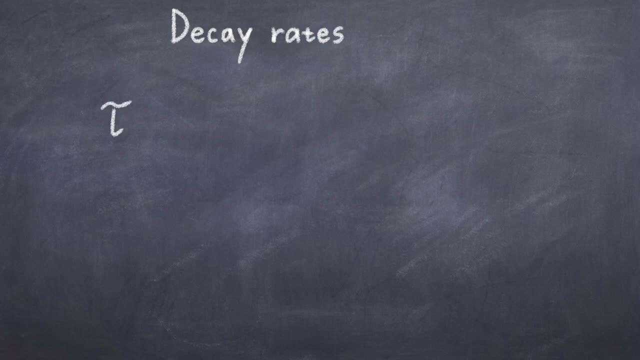 them, But how do we compare them to reality? How do we get from theory to a result which we can test in experiments? In particle physics we can measure two things: decay rates and cross-sections. Decay rates are rather simple, and we denote decay rates with capital gamma. 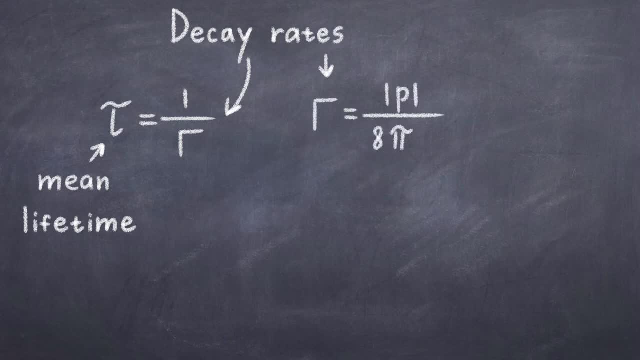 We simply figure out how much of some particle decays From the decay rate. we can also find the mean lifetime tau. using the simple relation, tau is equal to 1 over gamma. The full map of how we calculate decay rates is rather complicated, so let's skip to the 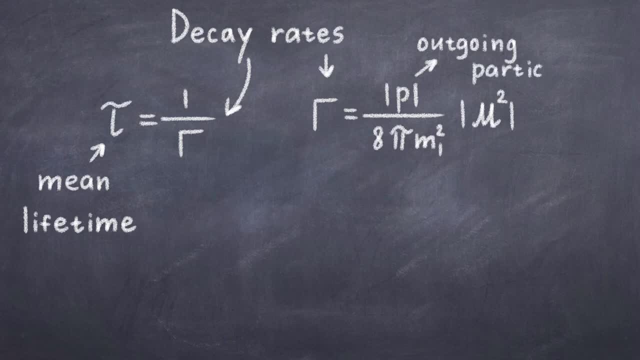 results and take it from there. For the simple case where some particle decays into two different particles, the decay rate is: gamma is equal to the absolute value of p divided by 8 pi m1 squared. A simple equation for this, therefore, is the following: 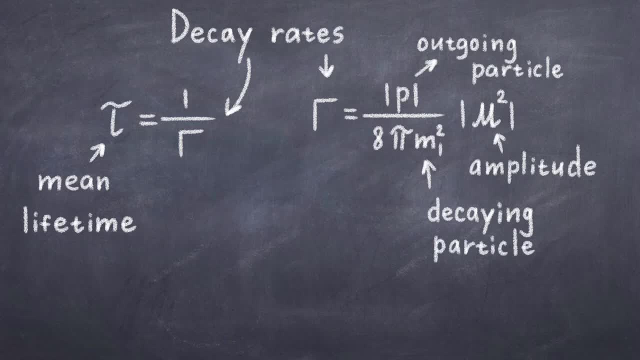 P divided by 8 pi m2 squared, B divided by 8 pi m2 squared, and all of that multiplied by the amplitude squared, where the absolute value of p is the momentum of either of the outgoing particles. We also have the dimension of the particles which decays, called m1,. 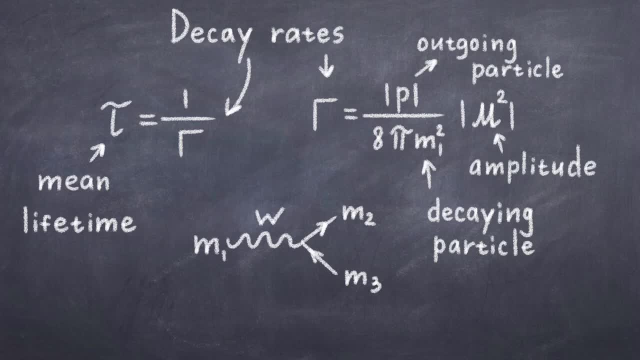 and the amplitude of the process m. This part is calculated using the Feynman rules, as we discussed in the previous video. A real-life example of this process could be the decay of the W boson. The other thing we can look at is the cross-section of a scattering process. 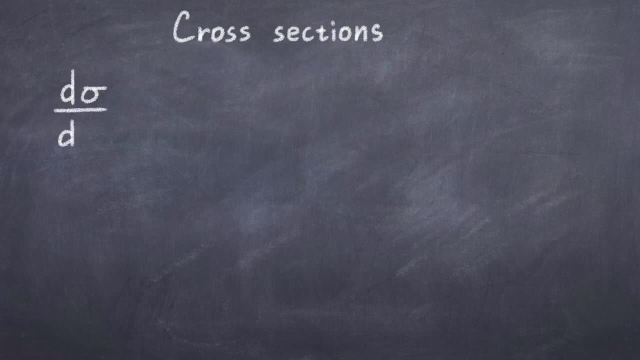 Since this process naturally involves two incoming and two outgoing particles at least, such processes are more complicated. In particle accelerators, one can smash particles together and make experiments regarding the cross-section of a process. It is often easier to work with the differential cross-section of a process. 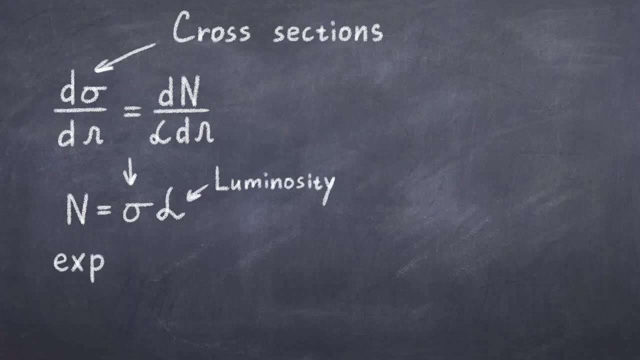 and this we write as: d sigma divided by d omega is equal to dn divided by l d omega, where the script l is the luminosity and dn is the number of particles and d omega is the solid angle of the detector and, of course, sigma is the cross-section. 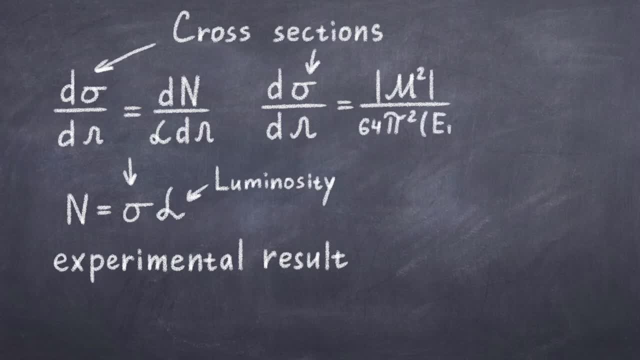 If we could completely surround the process with a detector, this would reduce to n. is equal to sigma l, where the event rate is equal to the cross-section times, the luminosity For the scattering process of two different incoming and outgoing particles. one can obtain the theoretical result using the following equation: 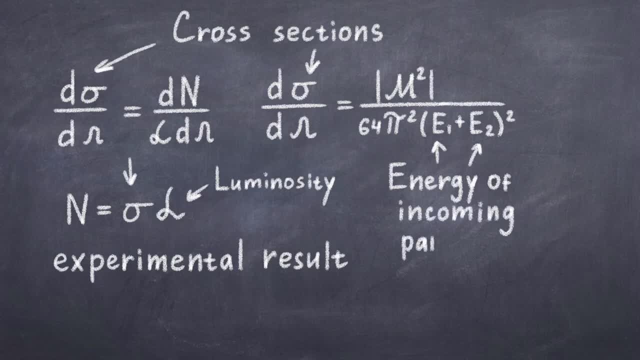 d sigma over d omega is equal to The amplitude squared divided by 64 times pi squared, and, in parenthesis, the energy of particle 1 plus the energy of particle 2, that squared, and then all that multiplied by the momentum of the outgoing particle divided by the momentum of an incoming particle. 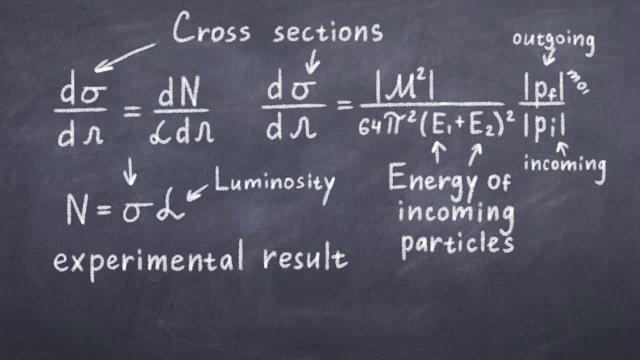 where E1 and E2 is the energy of the incoming particles respectively, We again have the amplitude, which must be calculated from the relevant diagrams using Feynman rules. The PF and PI is the momentum of either of the outgoing and incoming particles. 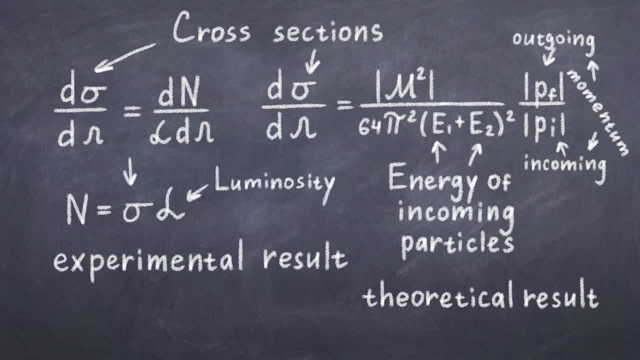 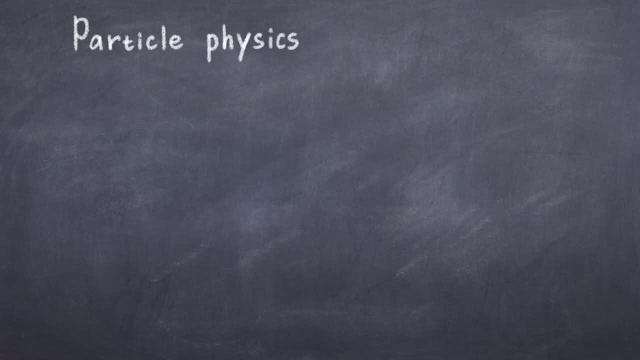 One can thus compare the experimental and theoretical result to check if the theory holds, which it generally does. In this video we have discussed a lot of different aspects of particle physics. The conservation of quantum numbers is deeply rooted in the math of the standard model. 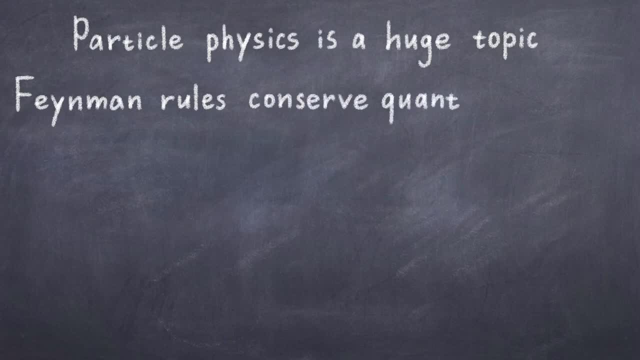 and in the videos about the different forces, we learn to master each of the forces and its Feynman rules. We will also understand the that just by following the Feynman rules then we will actually automatically conserve the different quantum numbers. 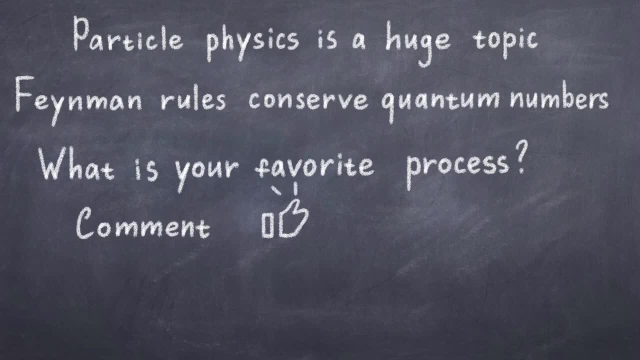 If you have some interesting processes which we should cover in an upcoming video, please put it in the comments with any other feedback. As always, I hope you have learned something new. If you did, please like and subscribe. Feel free to support me and buy me a coffee using the link in the description. 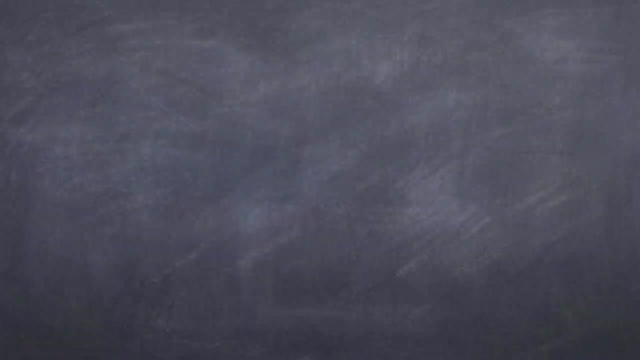 Stay tuned for more videos. Thank you for watching. See you in the next video.